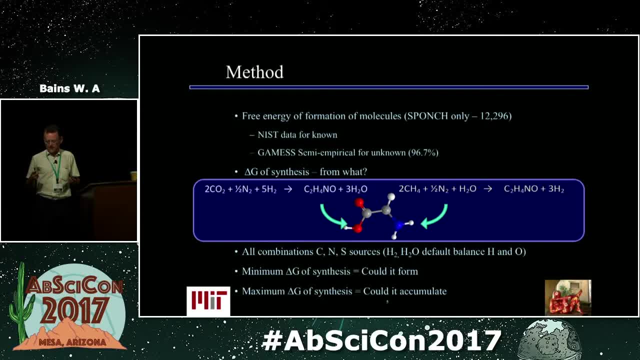 and we use the GAMES software to do that. Over 96% of the molecules in our database don't have reported free energies of formation, so we had to calculate enthalpy, entropy and specific heat capacity to work out the energy of synthesis. 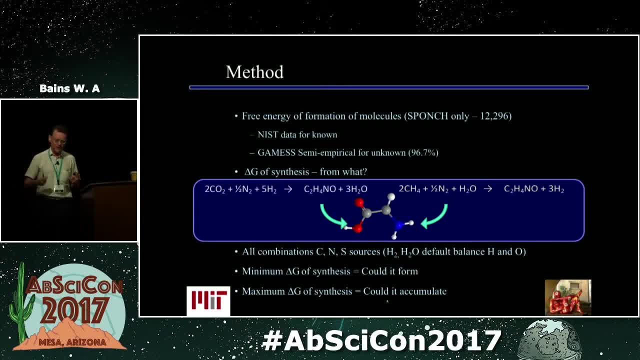 The other question is: synthesis from what? So? volcanoes put out a lot of gases and you can assemble them in different ways to make a molecule. So, for example, this is glycine, and you can make glycine by this reaction here, in theory, 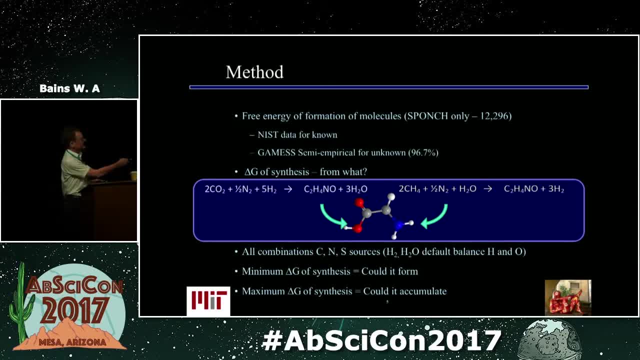 Okay, I'm not saying how it happens, Or from this one here, and these are different gases and hence we'll have a different free energy of formation. And how do you compensate for that? Well, you don't. You look at all of them, all combinations of the different volcanic gases. 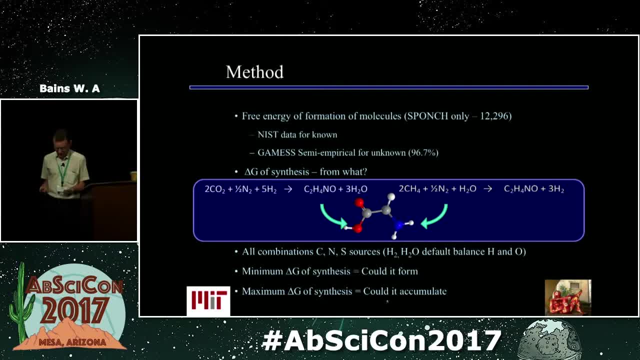 CO2, methane, nitrogen, ammonia and so on, and say what is the maximum Free energy? and that's the sort of ultimate limit of the minimum which suggests that this might happen in a volcanic system. So this is the sort of data we get out. 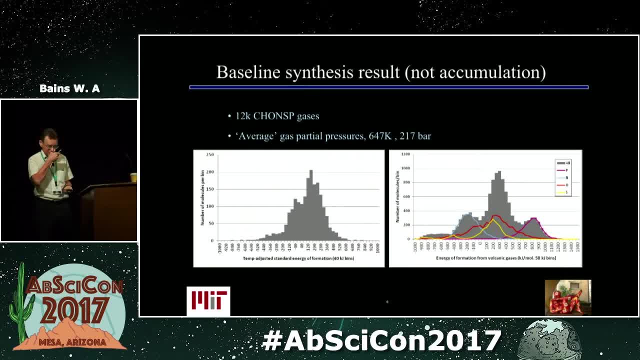 This is the number of molecules produced out of our database and this is the free energy of formation from elements in their standard state. There's quite a spread, but it's not terribly interesting because the elements are not in their standard state in volcanic gas. 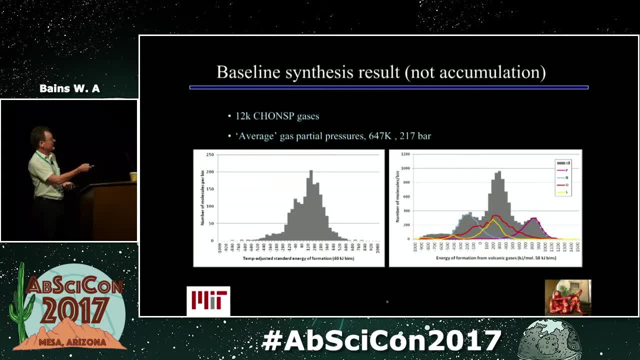 This is synthesis from volcanic gas. This is the number of gases. over here Again: number of gases and free energy of formation. Anything lower than zero means that's a negative free energy of formation. That means that the reaction as modeled here is thermodynamically favored. 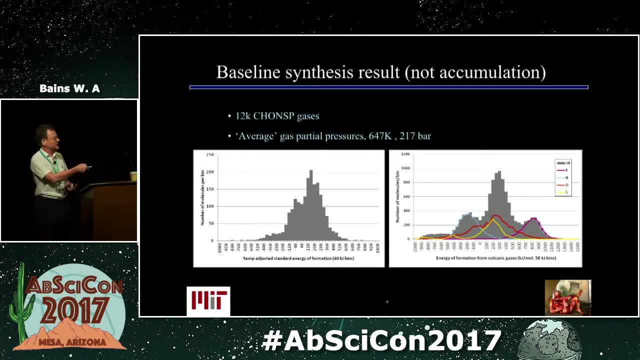 Quite a big spread and some obvious sort of bulges and humps in the curve. These guys over here are mostly compounds with phosphorus atoms in. These guys over here are mostly compounds with nitrogen atoms in which is interesting and we haven't followed up on that yet. 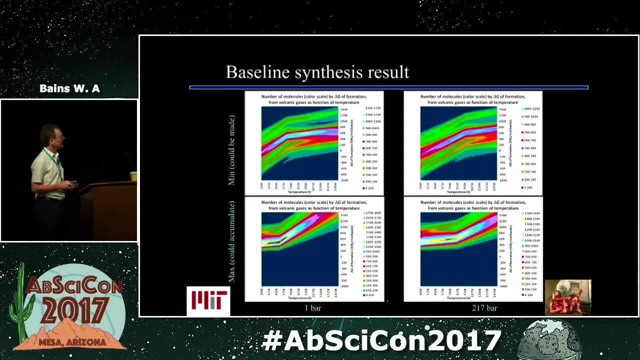 I said work in progress, okay, And you can do that for all temperatures. So that was just one temperature and one pressure. You can do that for all temperatures and a variety of pressures. So here we have temperature and here we have free energy of formation. 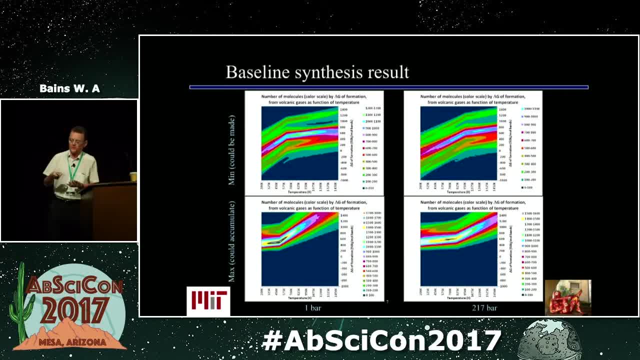 and the color scale here is the number of molecules falling into that free energy range for that particular temperature, And those look very pretty and they tell you that as you increase pressure from one bar here to 17,. this is arbitrary, by the way. This is just the critical pressure of water. You get more molecules that are likely to be formed thermodynamically. In other words, it's lower down the scale. The maximum value is higher than the minimum value. Always nice to have that sort of check in your software. 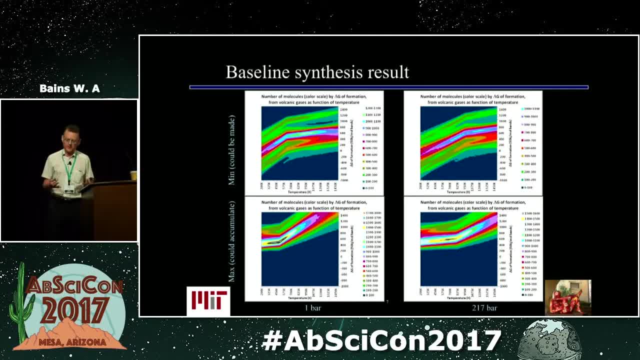 As you increase the temperature, the number of stable molecules goes down, And all this is totally expected. What isn't expected is this sort of kink here in the curve, and that's where it becomes thermodynamically favored On the right to make the molecules from methane. 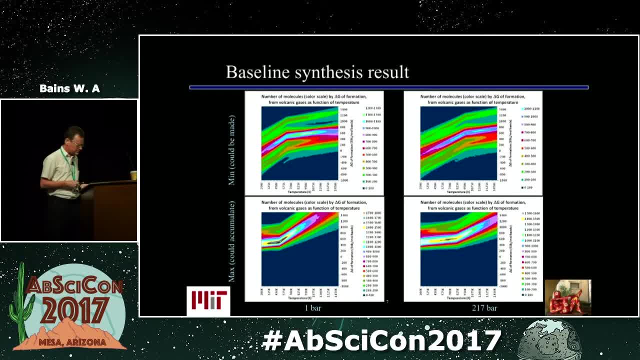 and on the left to make them from carbon dioxide and hydrogen. This can be done for everything. and then what we ask is how many molecules fall below delta? G equals zero here, In other words, are thermodynamically favored under these conditions, And that's great. except these conditions are sort of average volcanic gas. 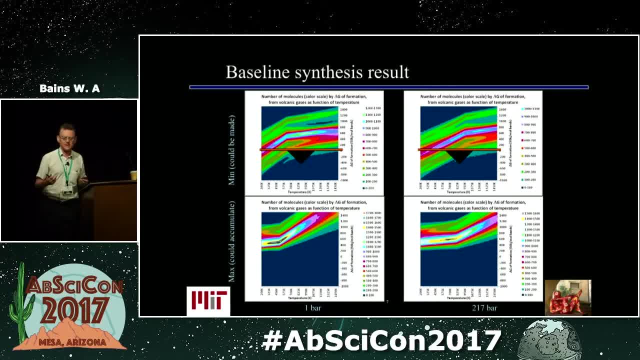 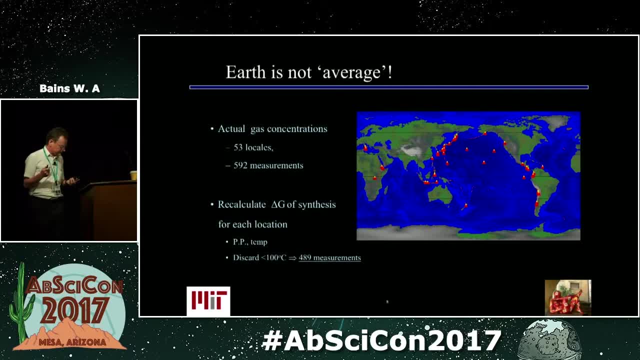 So if you look up in an atmospheric chemistry book what gases the volcanoes put into the atmosphere, and they come up with a number that is an average. Earth is not an average. So to try to get a little bit nearer to what the Earth actually does, 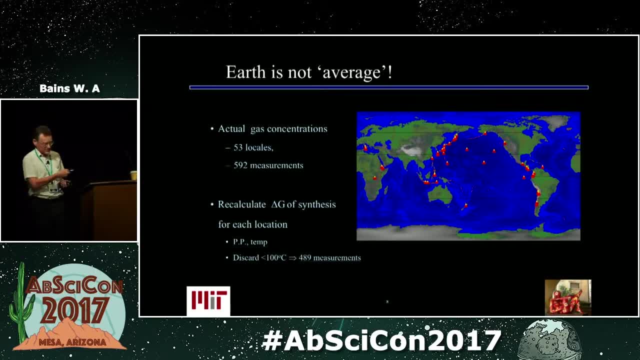 we looked at actual volcanic locales- 53 locales, around 60 different papers recording nearly 600 measurements of the actual gases coming out of the Earth- and did the modeling with that: The partial pressure of gases at these locations, the temperature at them. 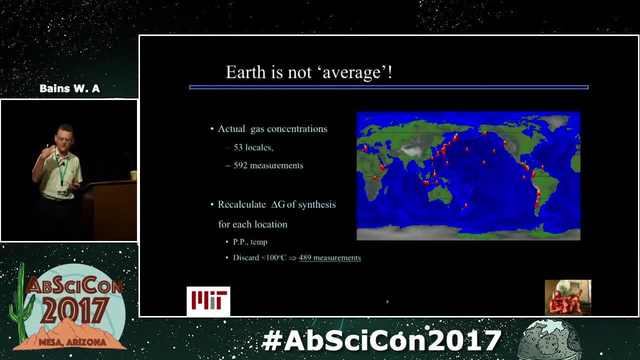 we discarded the ones below 100 degrees because this is a gas phase, not a gas liquid phase. The issues with that is, of course, that not all gases are measured at all locations, So we had to fill in the ones that weren't measured. 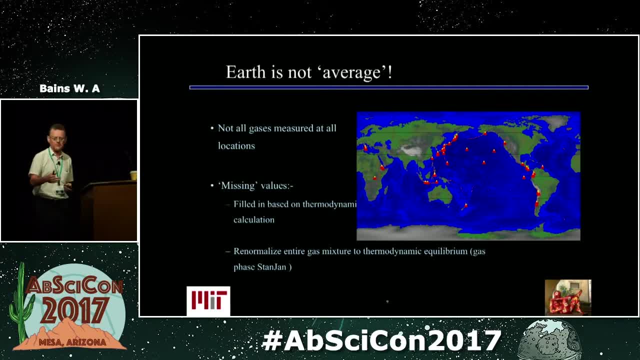 and there are two ways of doing that. You could do a thermodynamic model of that gas or a thermodynamic model of the whole system, and that gives slightly different results, which we're still working on. So this is the sort of result you get. 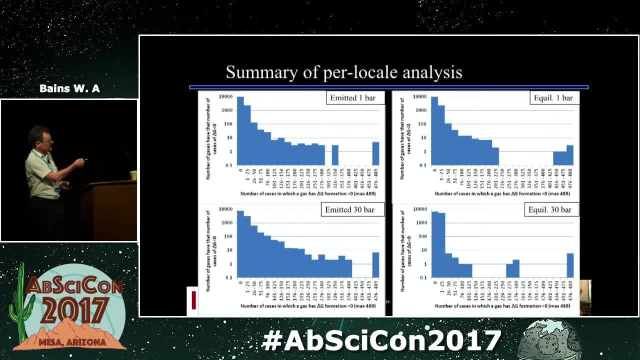 This is the number of volcanic sources out of that collection of 53 locales, or 487 measurements at which a gas is thermodynamically favored to be produced, In other words, delta G formation synthesis from those gases: less than zero. 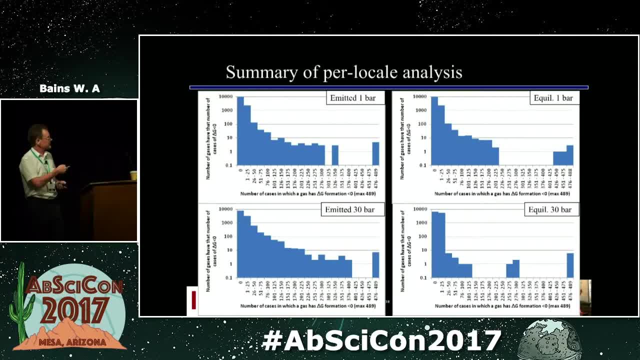 And this is the number of gases for which that number is right. So over here this is one bar, that's 30 bars, because I'm just going to do 1 and 30 and 1000, but 1000 turns out to be on the slide over there. 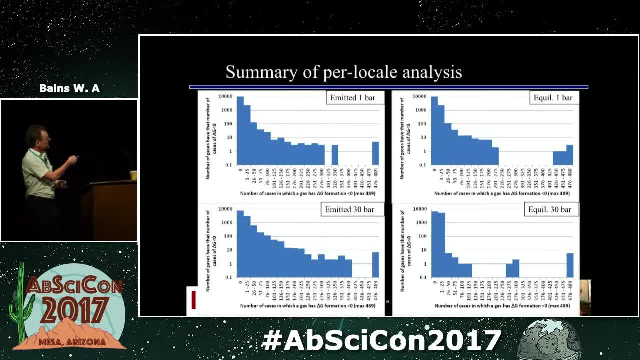 so you know, And the large majority of the gases are not produced in any volcano. Good, they're not likely to be false positives. As you increase the pressure, that number goes down. There's a small number that's produced virtually everywhere. 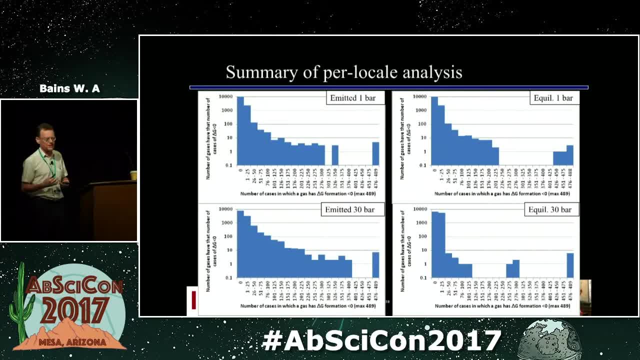 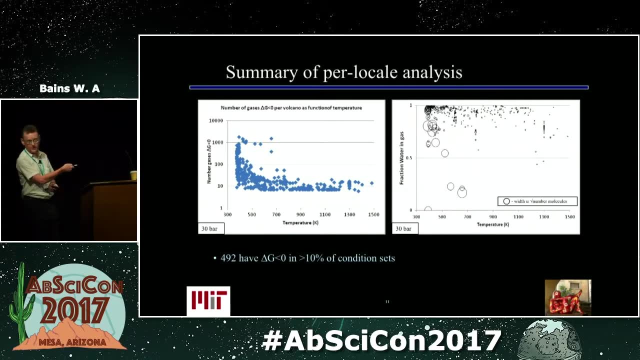 and that includes things like sulfur dioxide, carbon dioxide, hydrogen sulfide, which we know volcanoes produce. So again, that's nice. Okay, that's enough of that one. This is the same data plotted a slightly different way. This again, this time, is temperature along here. 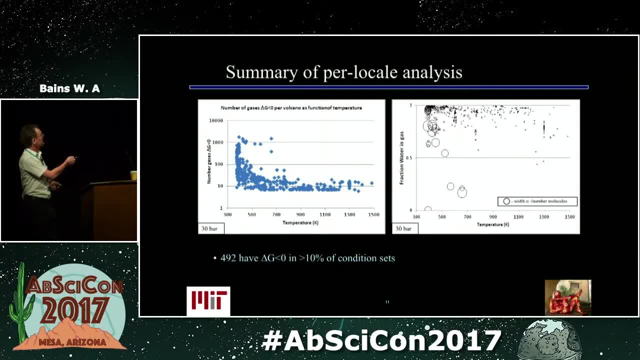 Each of these dots is one volcano, and this is the number of gases produced by that volcano, And it drops off with temperature. as you'd expect, There's really weird outliers up here, though, And if you plot the data a slightly different way, 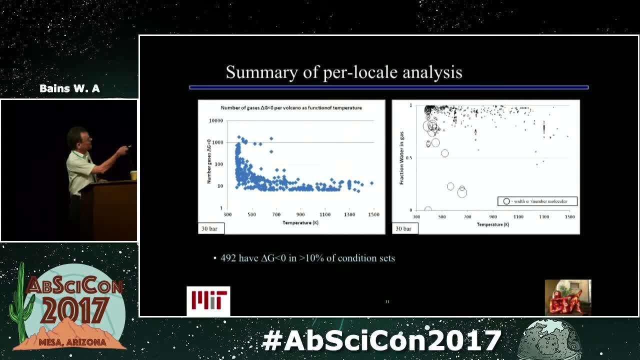 so this is temperature again along here, but fraction of water in the gases. Your average fumarole or volcanic vent produces 90, 90, 95% of water as the gas. Some of them produce much less. And these large circles here? size of the circle is proportional. 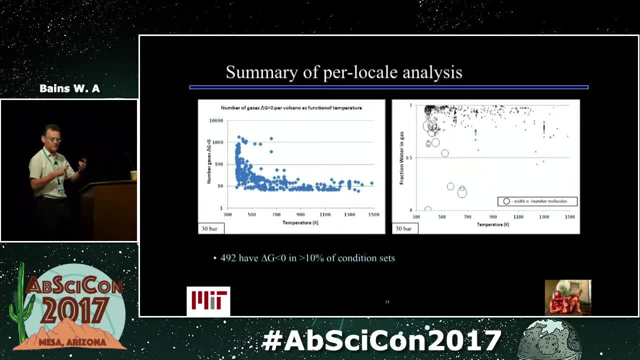 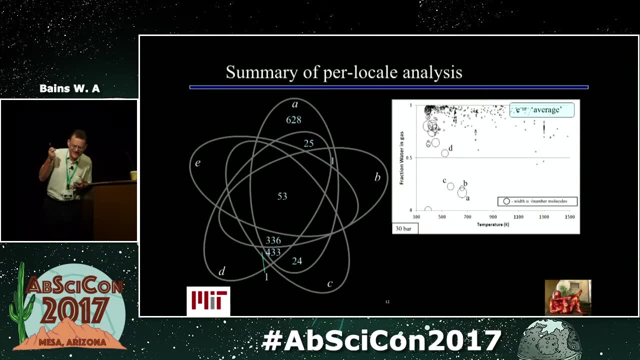 to the number of molecules being produced under this thermodynamic modeling in the system. The dry gases down here seem to produce a lot more potential gases. Okay, But- an important point to remember- these are not the same gases in each volcano, So I've looked at these four examples here. 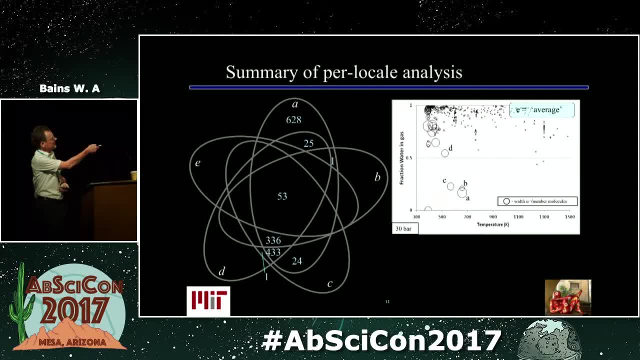 and a sort of average one up here, And this is the number of gases produced by those models- to be produced by those, I should say- and how many are shared between them. So system A, here the 628 molecules we predict as having a negative free energy of formation. 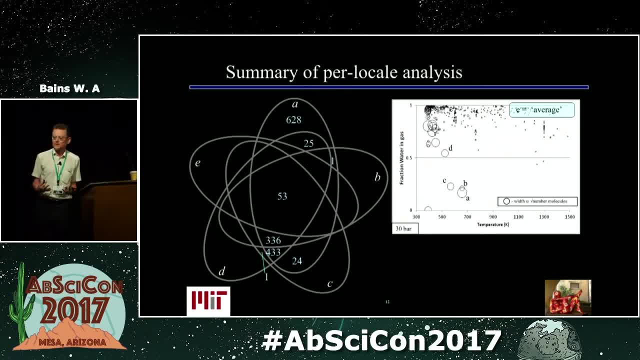 that are not formed in any other system And there's a tweak to this because actually A, B, C and D are all the same volcano. They're all the Lascar volcano in Chile, at different times. So different places, different times, different volcanoes. 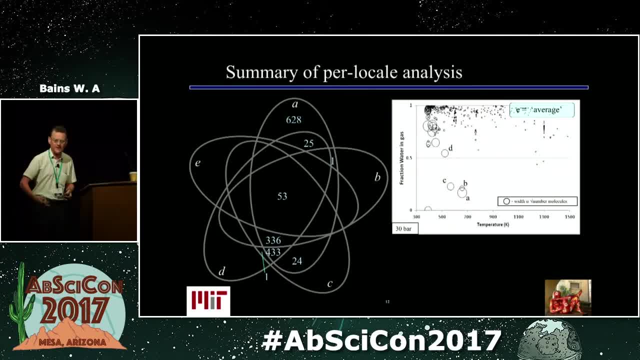 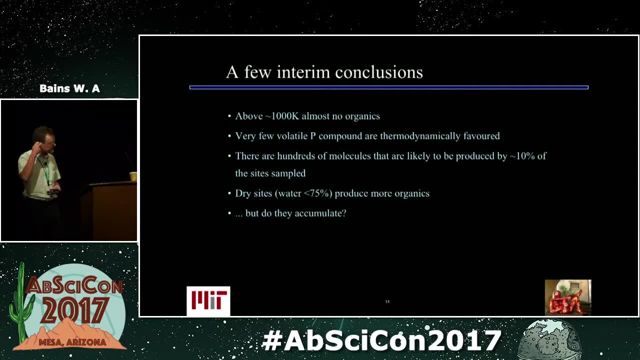 all produce different materials And we're going to have to capture this if we want to model this on an exoplanet. Okay, So interim conclusions. As you'd expect, above 1,000 Kelvin you produce very little complex molecules. 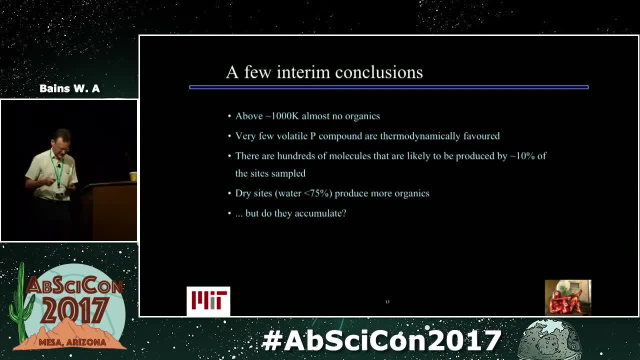 They're all the obvious volcanic gases. I was going to put something fairly rude up here to say, well gosh, isn't that surprising? But I didn't. Phosphorus compounds: very few volatiles. If you see a volatile phosphorus compound in an exoplanet atmosphere. 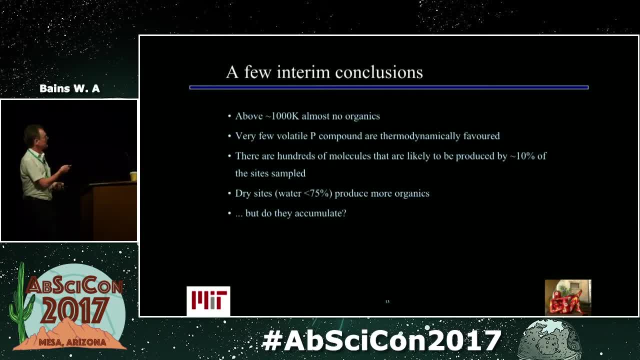 you say: wow. Lots of molecules likely to produce Dry sites produce more. What we don't know yet is whether they accumulate Biases in the data. Phosphorus is a problem, And if anybody wants to ask how I deal with phosphorus, 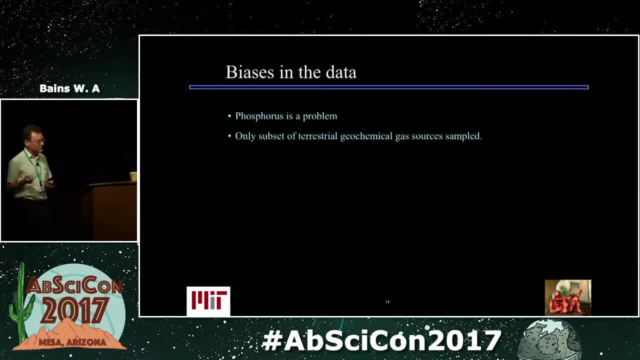 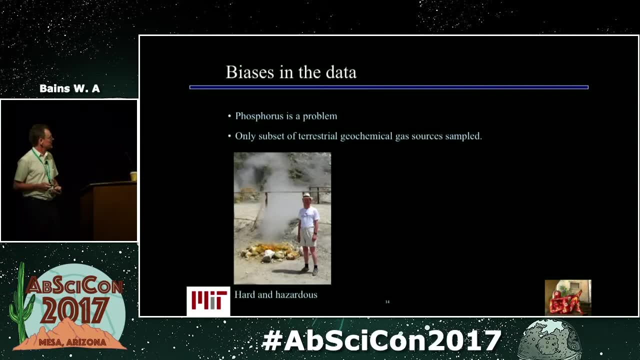 I will tell you either in questions or afterwards. But the big problem is that these are a very biased set. They're biased because of volcanic gas samples And they're biased for a very simple reason. If you want to sample this fumarole here, 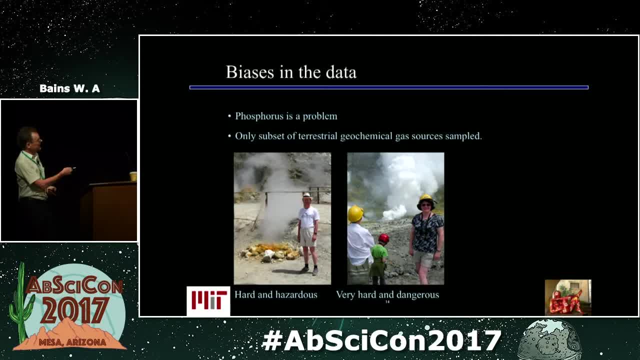 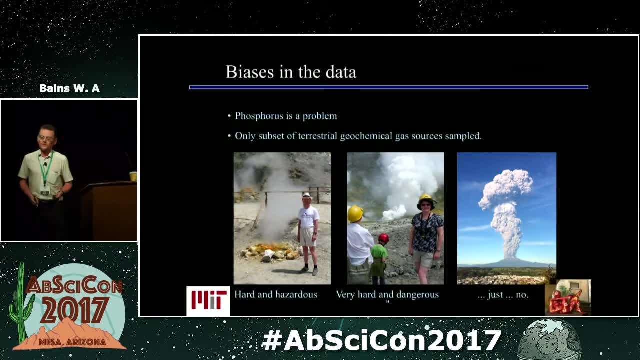 it's a bit hazardous but reasonably safe. If you want to sample this active volcanic crater here, it's really dangerous but possible. And if you want to sample this, well, frankly you just don't. But these sort of things put about a third to a half. 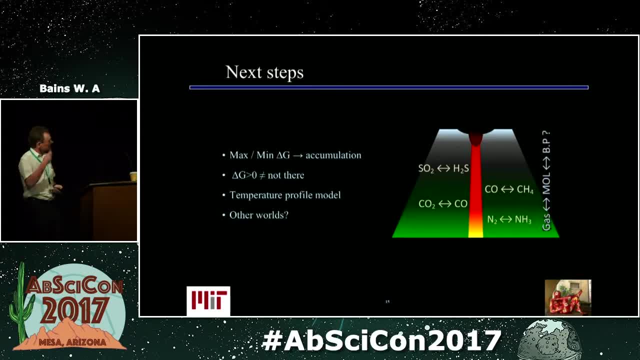 of all the volcanic gases in the atmosphere. So this is interim. There are a number of things we want to do next which I'm really keen to talk to people about, but particularly other worlds. what other volcanic gas models might be put into those worlds? 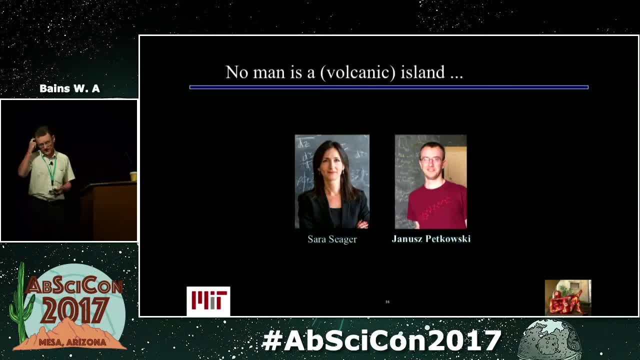 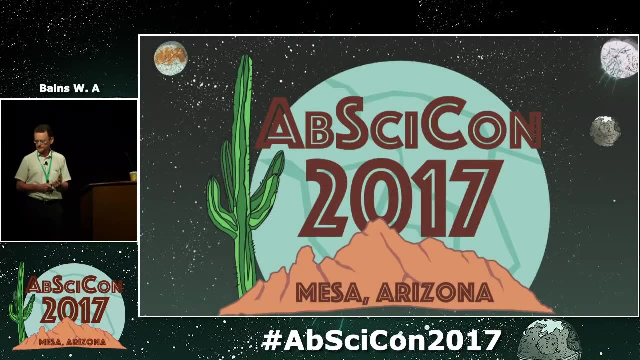 And that's it. Huge thanks to Janusz- I can't see you There you are- And Sarah, of course, who's been my sponsor in doing this for many years, And thank you for your attention. Thank you, We have time for a couple questions. 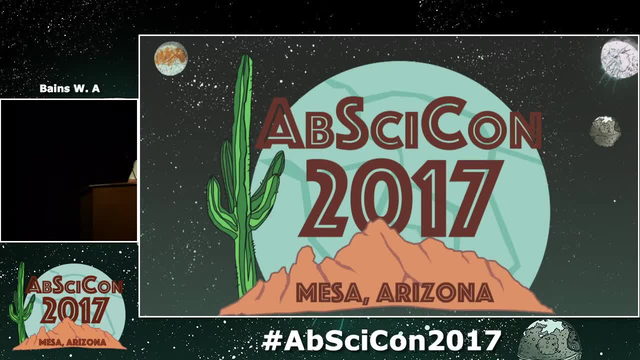 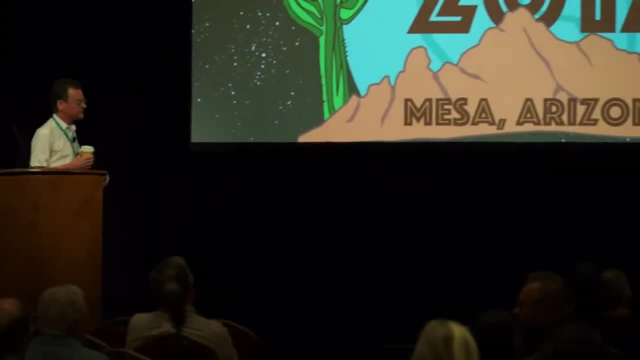 Excellent. That's all I'd like to see. So I'll ask a question if there are none. So you mentioned right there at the end other models for different types of planets. I mean, do you have any thoughts of where you're going to start there? 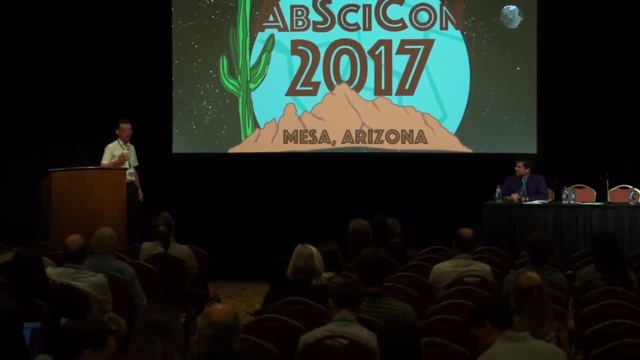 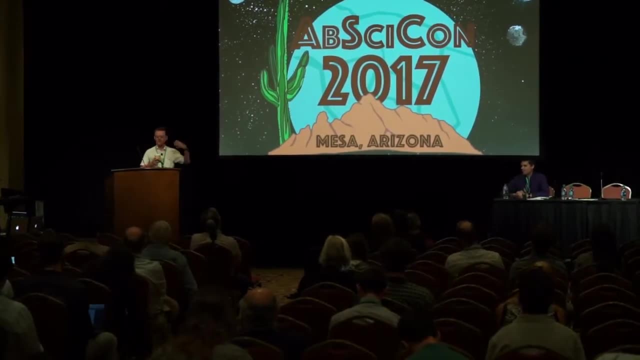 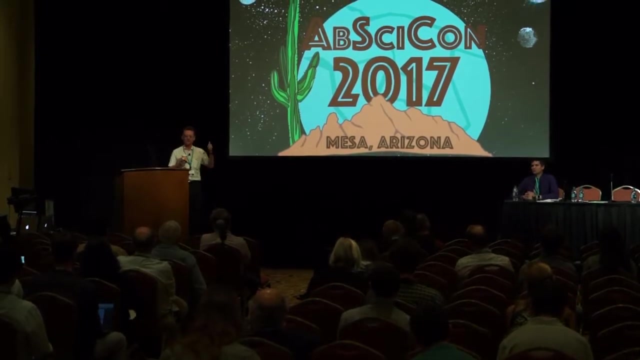 I'd really like to start on Io. Okay, I think Io is just fantastic, apart from looking at brilliant color, But it's a known body for which we know is very active and has a lot of volcanic activity Beyond that. I had somebody who told me that volcanoes and Venus have been detected as active, but how do you measure the gases in them? You need something where you can actually say what is the gas coming out of this and then plug that into these sort of calculations. So Io will be number one. 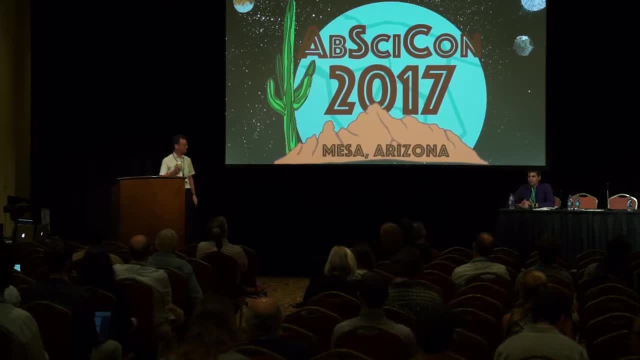 And then after that, you know the field's open. Thank you very much. Any other questions You have to go up to the microphone. unfortunately There's no one who's coming around with them, Hi. So my question is very similar to that. 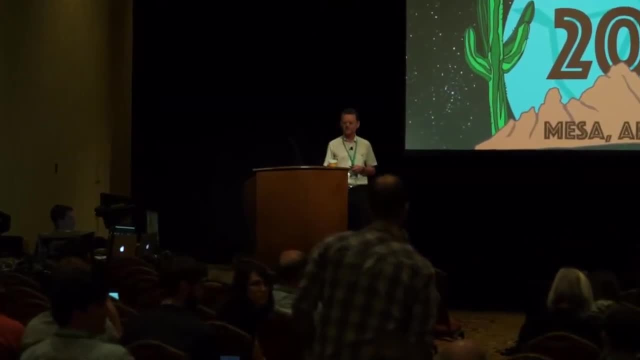 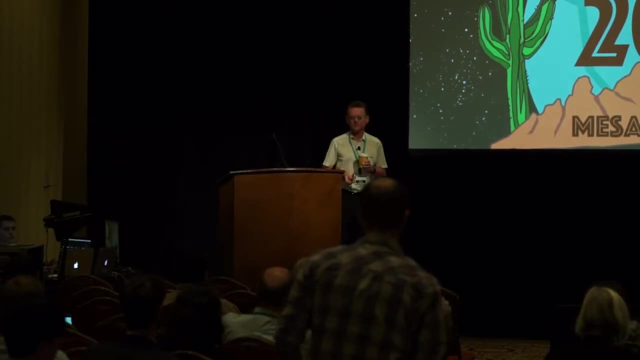 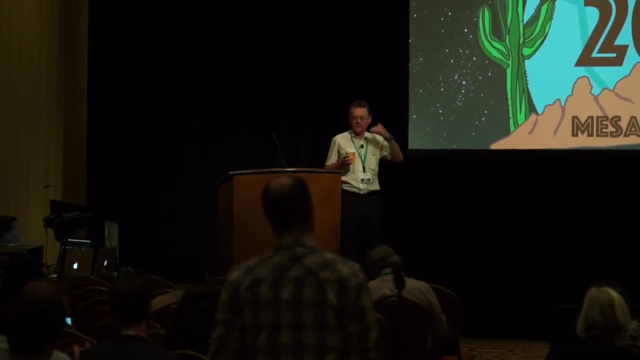 which is, we can find these volcanoes around other bodies and measure the gases, but what kind of lab work could be done to actually measure the gases in their free energies? Is that a viable avenue as well To So there's work to measure more gases? 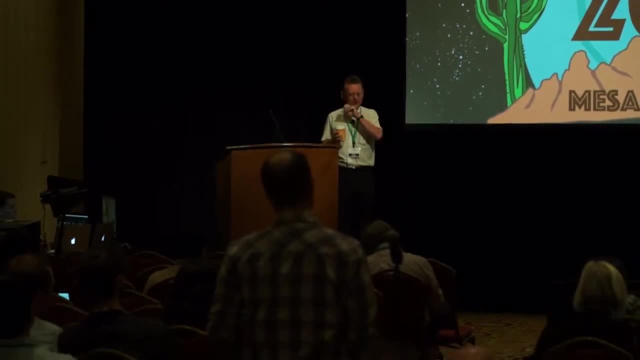 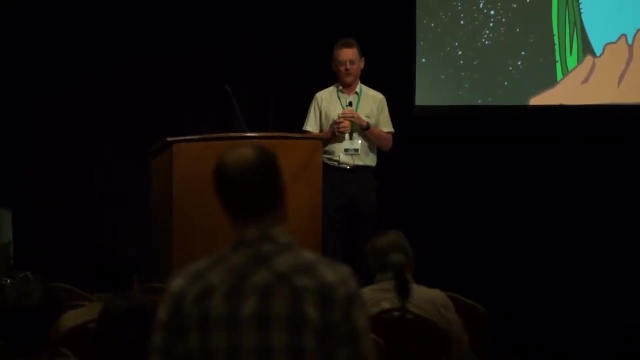 and to fill in all those gaps There's. A lot of this is based on calculated thermodynamic parameters and some of the calculations are quite badly off because if you compare them to what's actually measured, you know. I mean they're off by tens of kilojoules per mole. 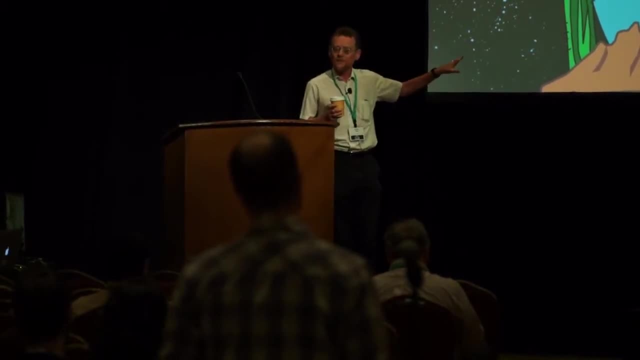 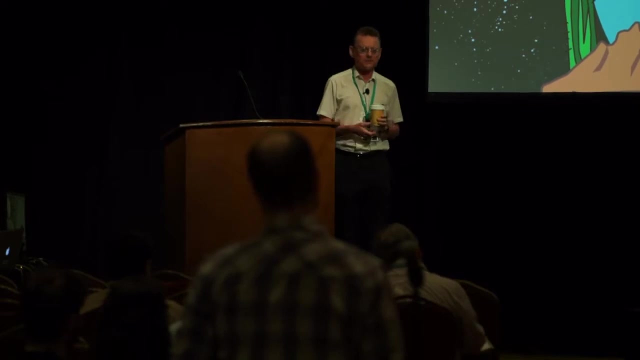 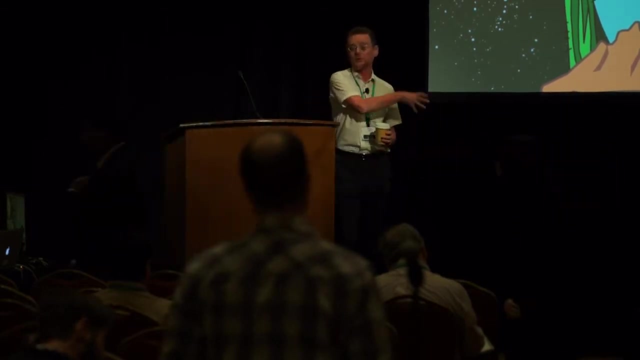 And so, as a first approximation, this is okay, but measuring those thermodynamic parameters would be really useful. The difficulty with this- and we talked about this at the Nexus seminar last summer- that doing those measurements and doing reaction rate measurements, which is also important for this. 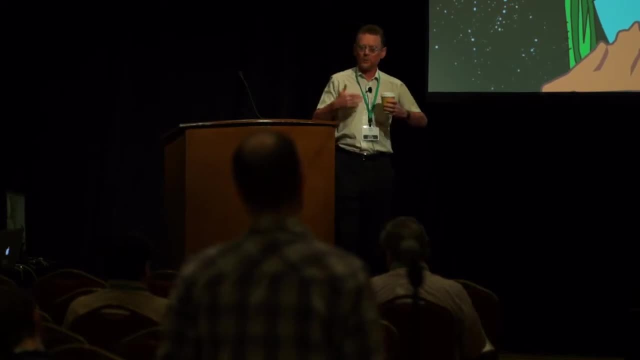 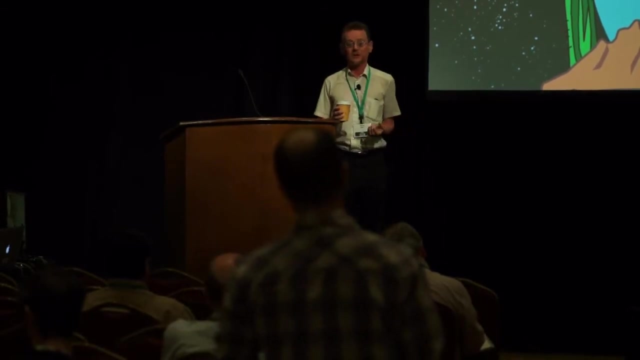 is really difficult, really time-consuming, and then once you've spent, you know, six months doing it for one set of chemicals, you get one data point in one database and no kudos at all. So there's a sort of risk-reward- time-reward imbalance there. 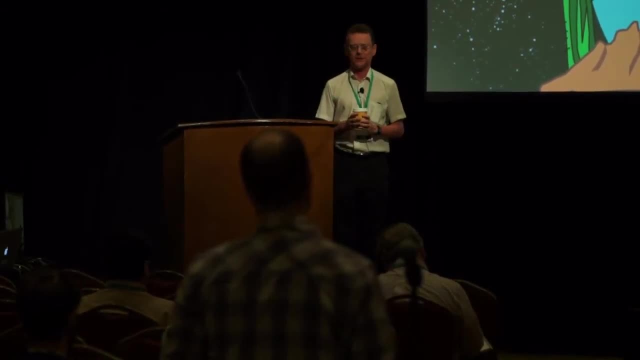 Don't know how to get around that, but if there's a technological solution around that, again really keen to hear about that. Thanks,